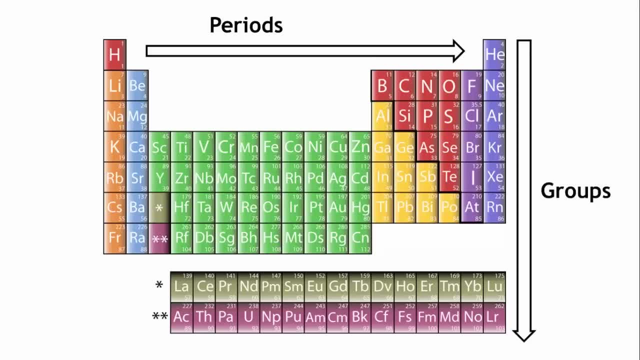 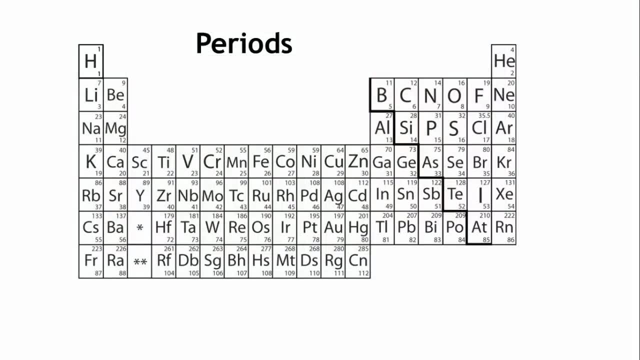 in periods and groups, going from the light elements at the top to the heavy elements at the bottom. The rows going across from left to right are periods. Elements in the same period all share something in common: They have the same number of energy shells. Each new period row. 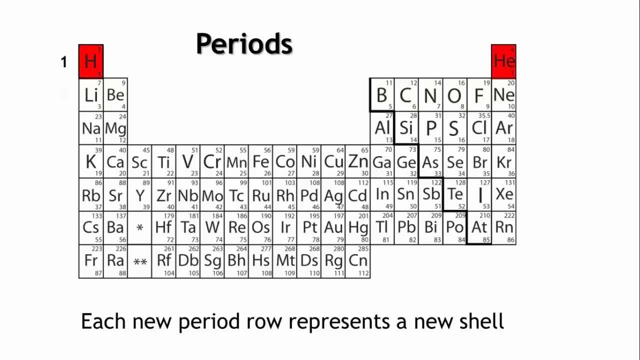 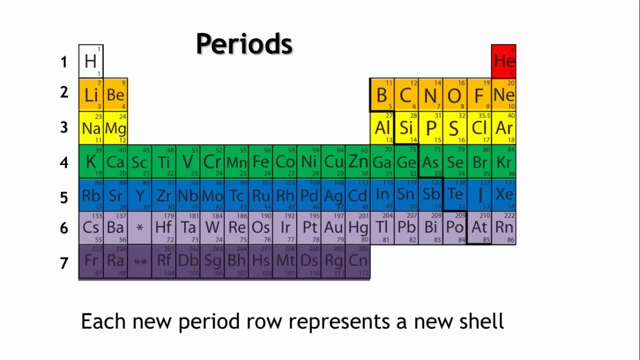 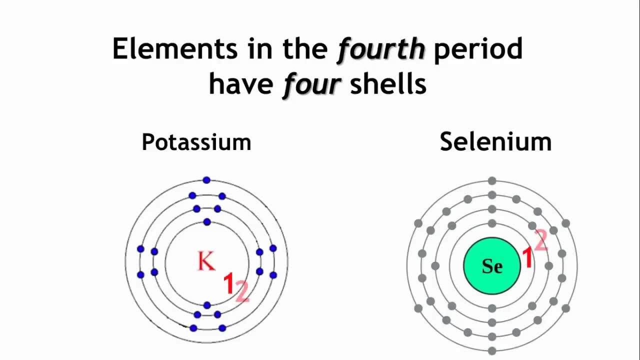 represents a new shell. Elements in the first period have one shell and as we go down, the shells increase. Hydrogen is in the first period. It has one shell. Potassium is in the fourth period and has four energy shells, as do all the other elements in this period. The columns going down. 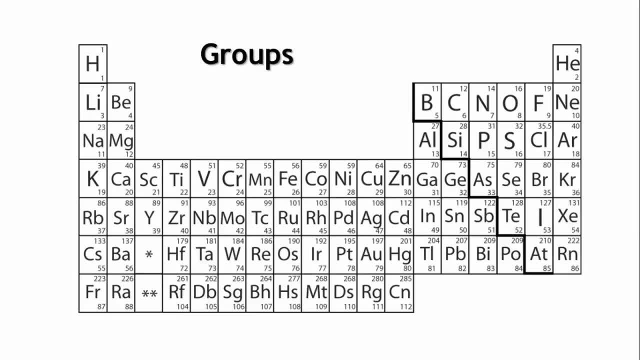 from top to bottom are the groups. Elements in the same group also have something in common. Elements in the same group have the same number of electrons in their outermost shell. The electrons in the outer shell are called the valence electrons. This just means that these 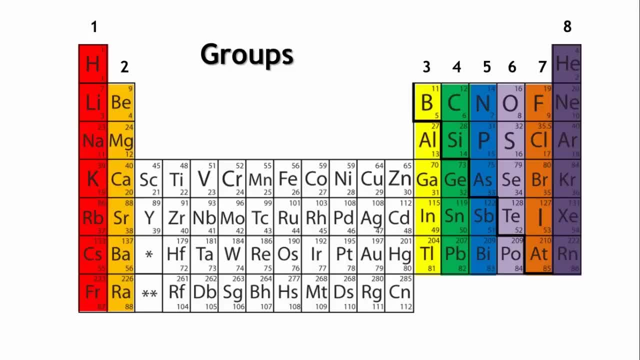 are the electrons available for reactions and bond formation. The number of electrons in the outer shell governs elements' reactivity, which is why elements in the same group have similar properties. The group number can tell you how many electrons are in this shell. 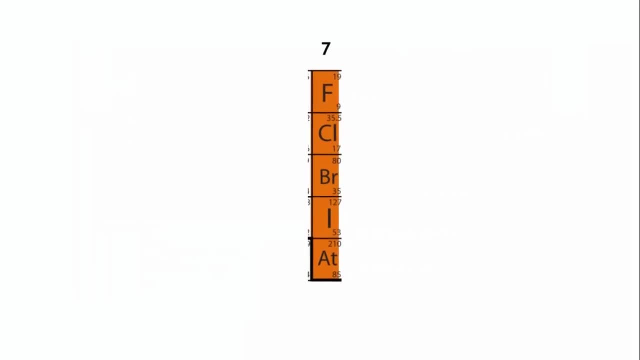 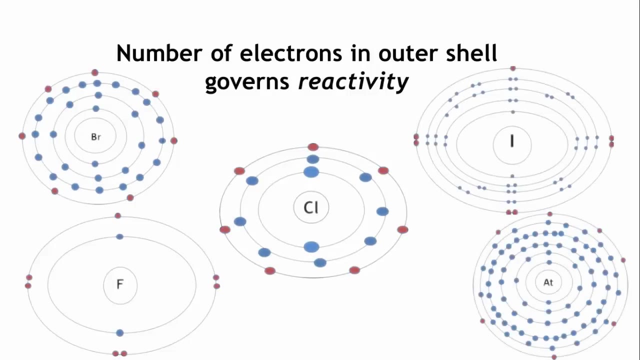 For example, let's look at group 7.. Fluorine, chlorine, iodine, copper, copper, copper iodine, bromine and acetine. They all have seven electrons in their outermost shell and all exhibit similar chemical characteristics. The properties show a gradual change going. 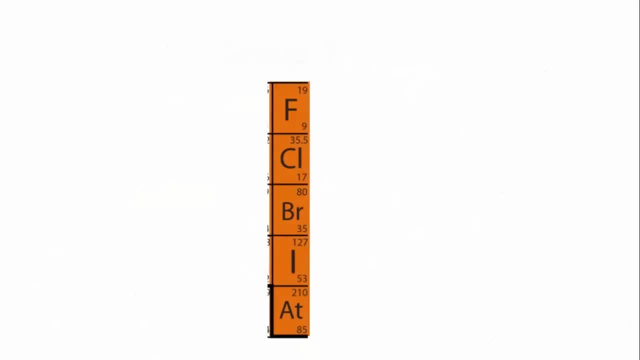 down the group as we go from period to period. So if we look at group 7 again, we can see that they are each in a different period in the periodic table, telling us that each element in this group has its outer electrons on a different shell. So chlorine is in group 7. 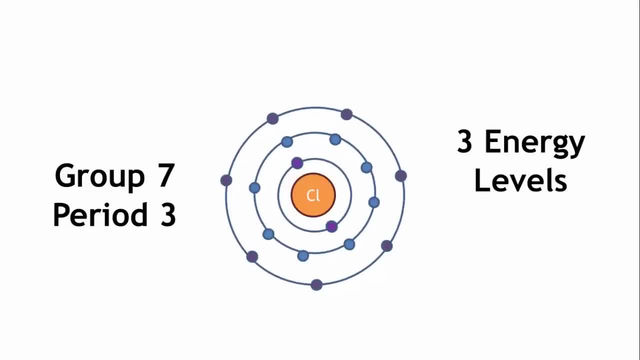 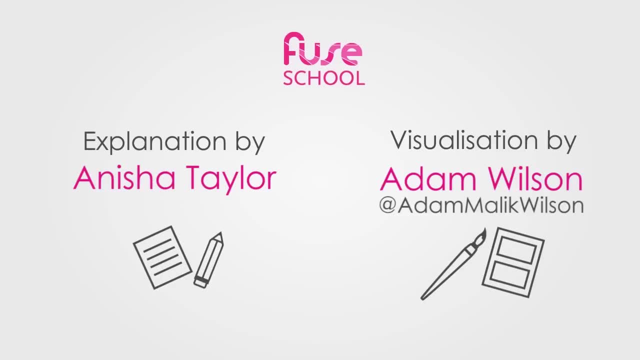 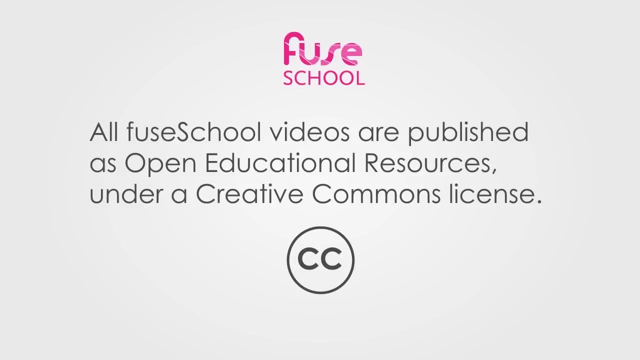 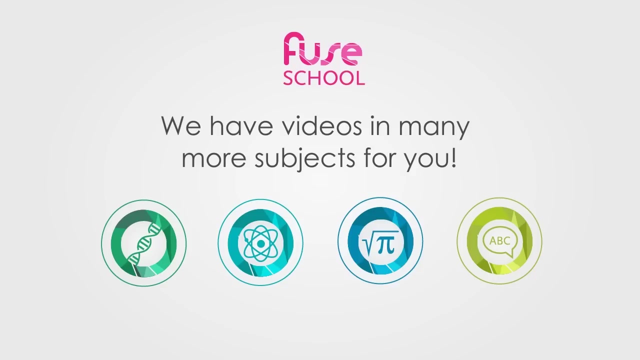 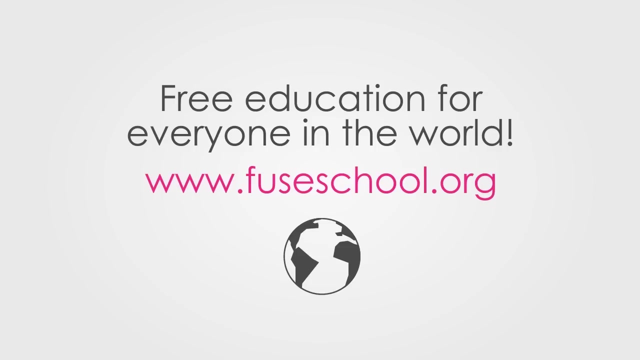 period 3. Therefore it has three energy levels with seven electrons in its outermost shell. So when this is a kind of a